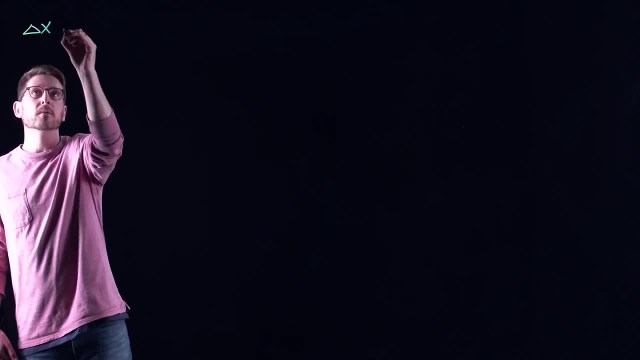 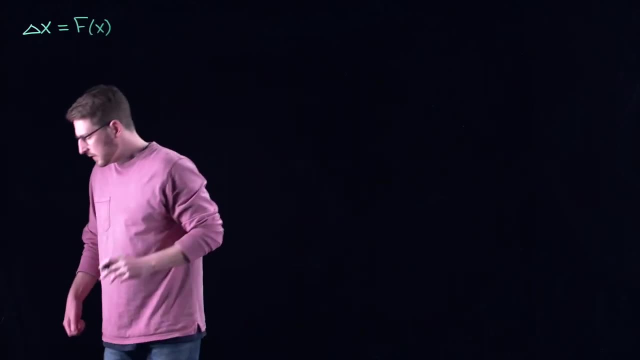 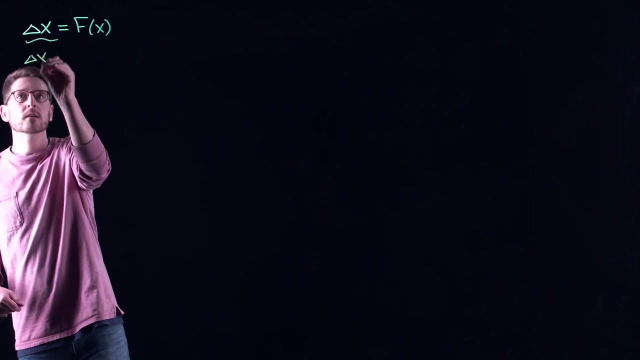 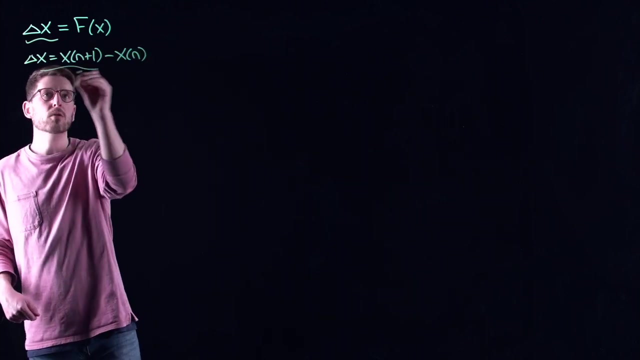 as the change in some state variable x is equal to a function of that state variable. Now, typically we like to actually open this up a little bit. Remember that the change here this is what you're doing next versus what you're currently doing, And so this typically gets opened up into a difference equation. 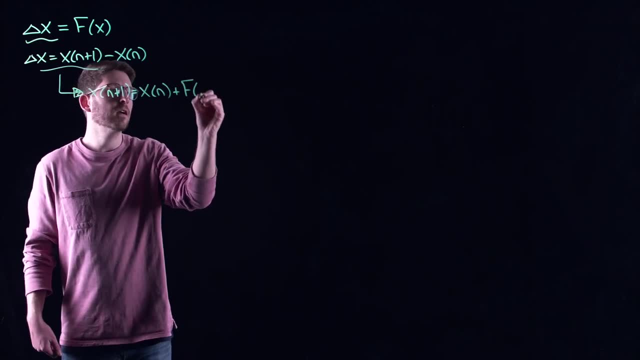 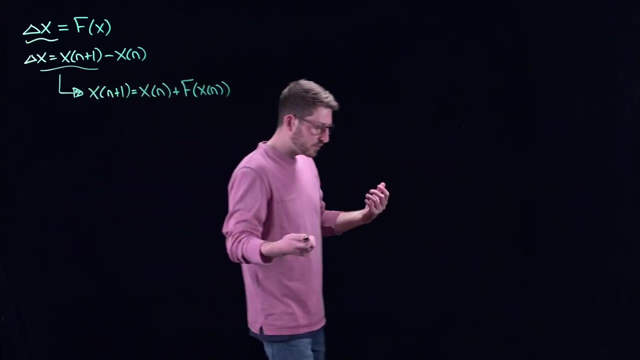 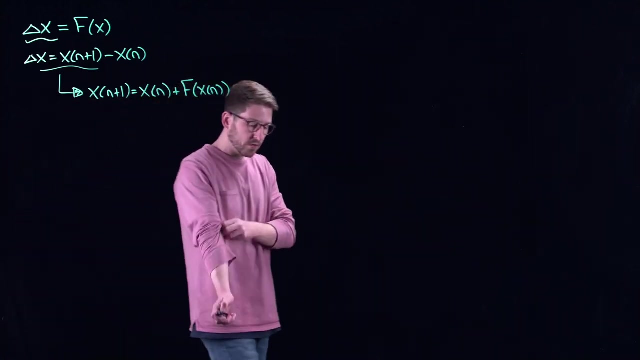 where we say: if we know what we're currently doing, then we know what will happen next. Things like Newton's method or gradient descent. these are examples of these kinds of difference equations, But of course we've seen over and over throughout this class that we can model. 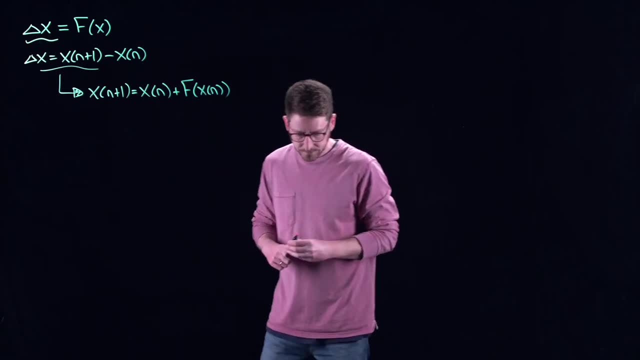 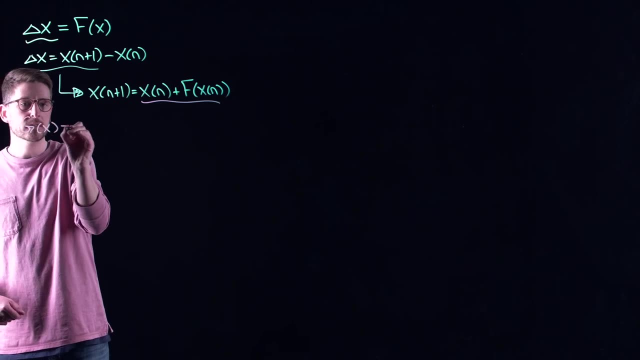 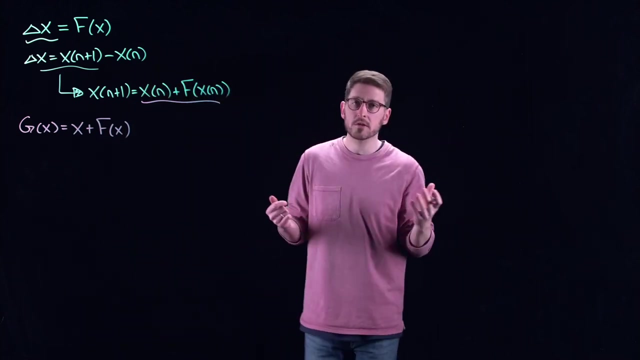 things like yeast populations through these types of models. Now if we call this whole piece right here g of x, so if we say g of x is equal to x plus f of x, we can do a similar process to what we've been doing with continuous time dynamical systems. 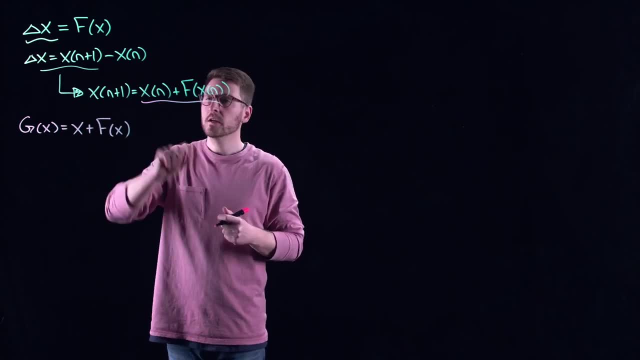 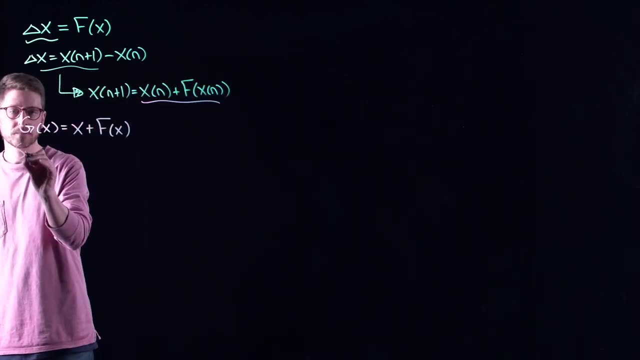 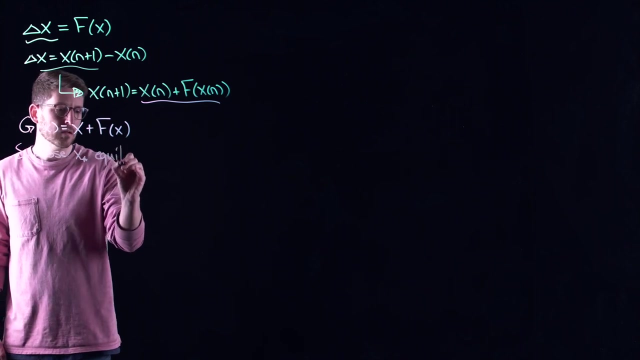 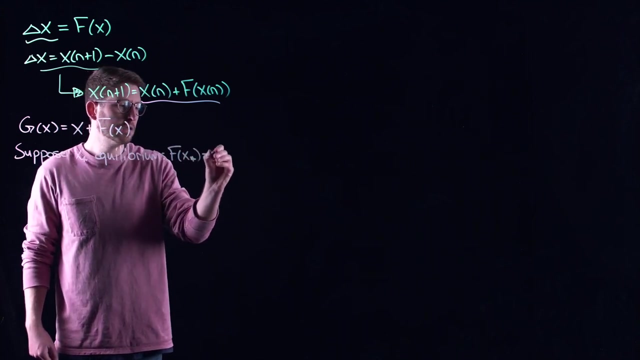 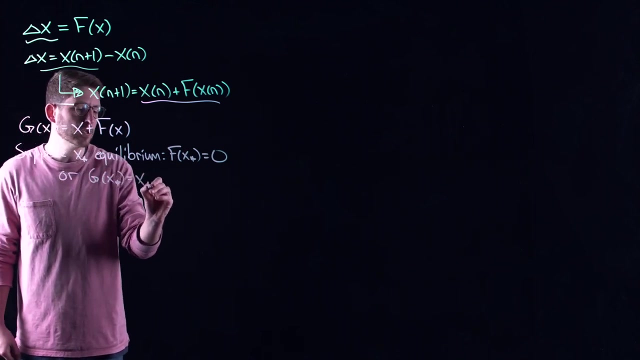 That is, we can linearize around a fixed point or an equilibrium for this thing. So let's suppose. so suppose x star is an equilibrium. Now remember: this means that f of x star is equal to zero, which is equivalent to saying g of x star is equal to x. Now, it's two different interpretations. 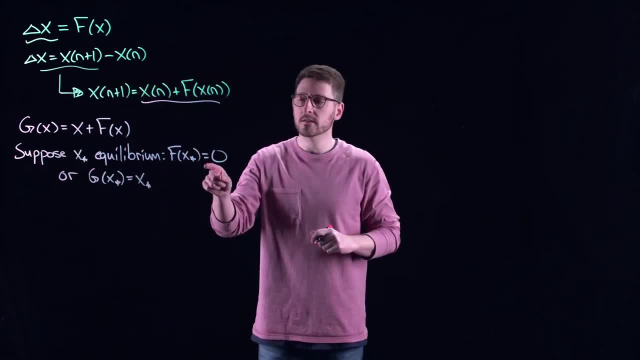 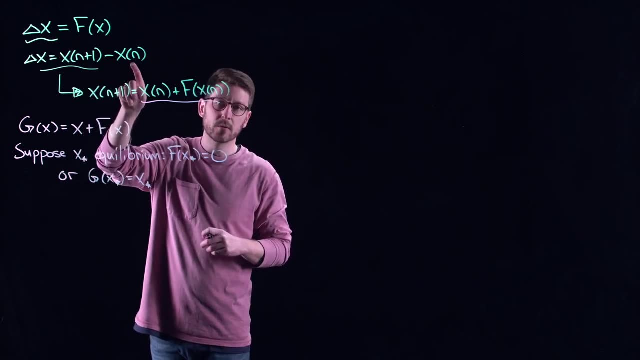 of exactly the same thing In the case where f of x star is equal to zero. that tells you that there's no change from step to step. That means that what you're doing next is the same as what you're doing now. Now, putting it in this interpretation of a difference equation where 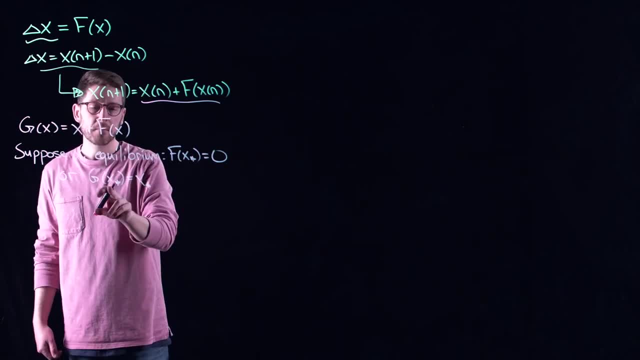 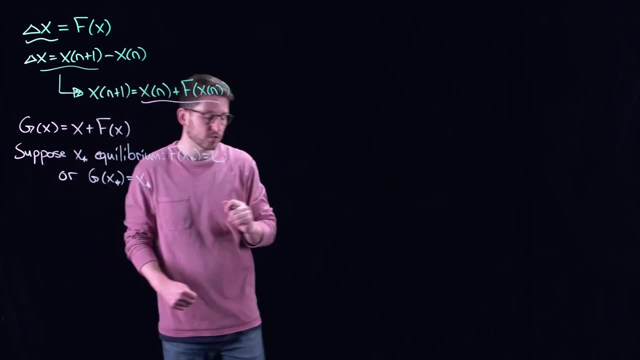 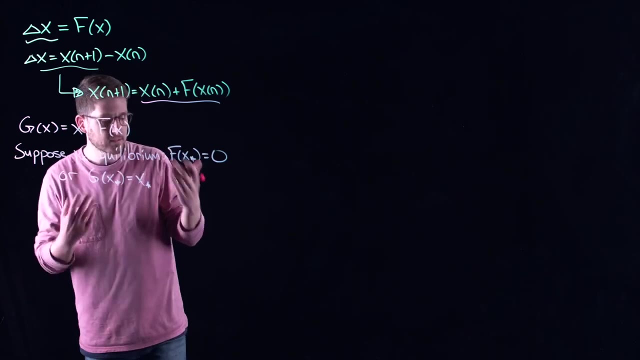 you're going based on what you have. that means that if you currently are at the equilibrium, you're going to stay at the equilibrium. So these are two equivalent views of the same thing, but, as I said, this is typically the more standard notation that you'll encounter, because things 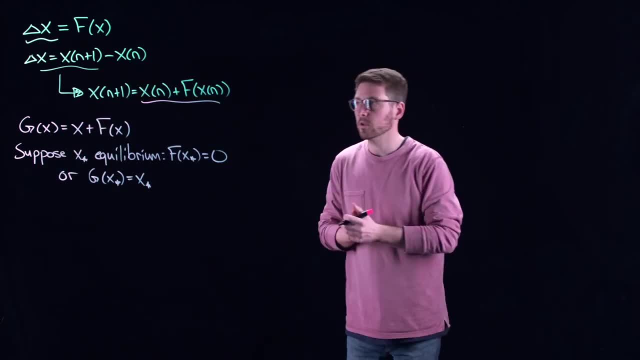 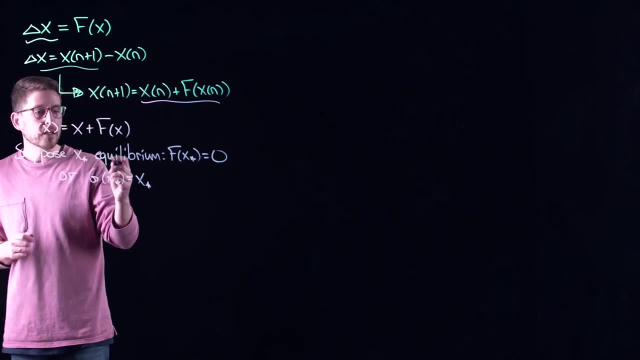 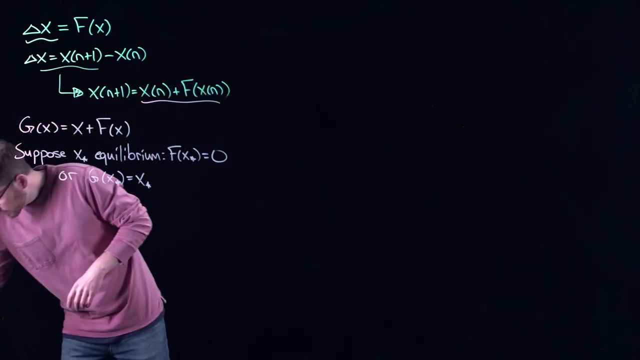 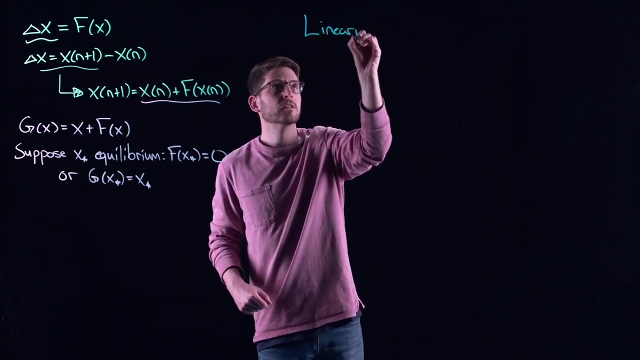 like Newton's method or gradient descent, even Euler's method that we'll explore in the next video. they all get put into this equation. Now, what we did with the continuous dynamics is we linearized. we took a Jacobian matrix about this steady state. We can do the same thing, So we have a linearized equation. So we say: linearized this. 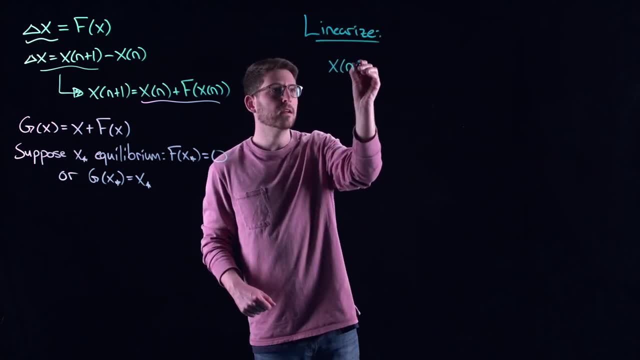 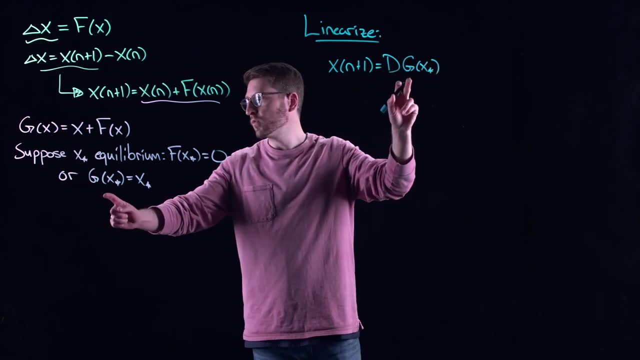 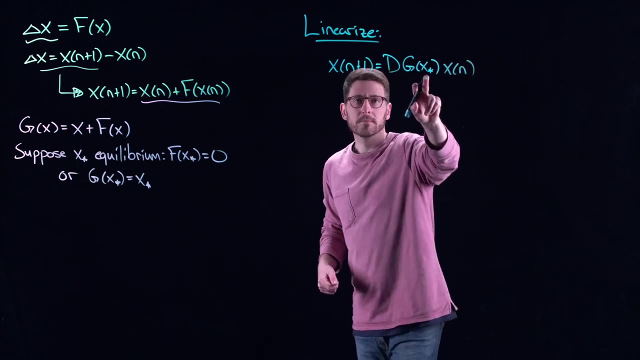 means compute the Jacobian and we would get an updating scheme that is the Jacobian matrix of my function g. So this is what we're going to do. So we're going to do a linearized equation. This is why I want to work with this g function here at the equilibrium. Okay, so this is a completely 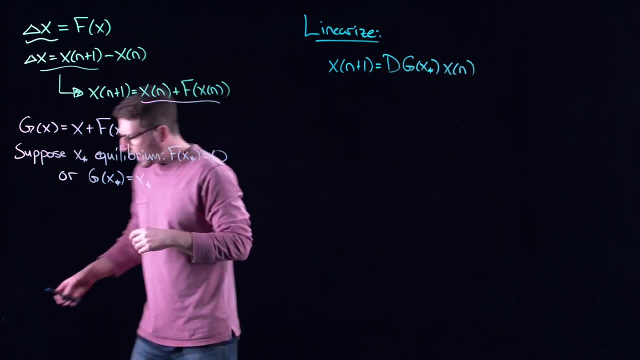 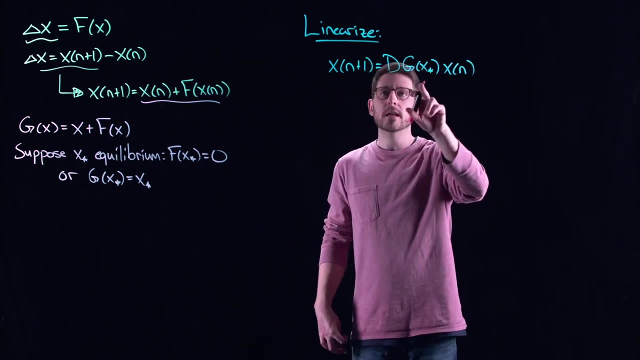 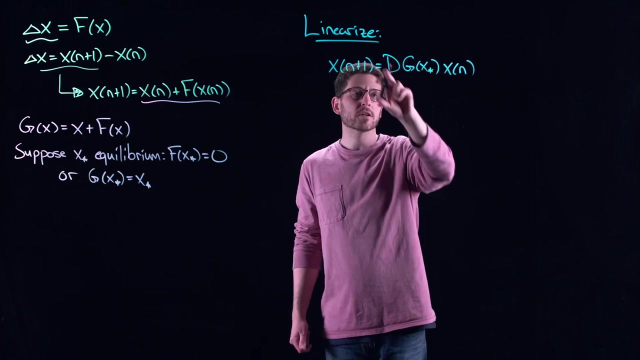 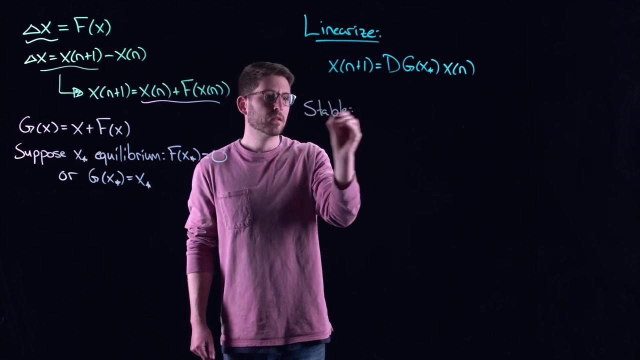 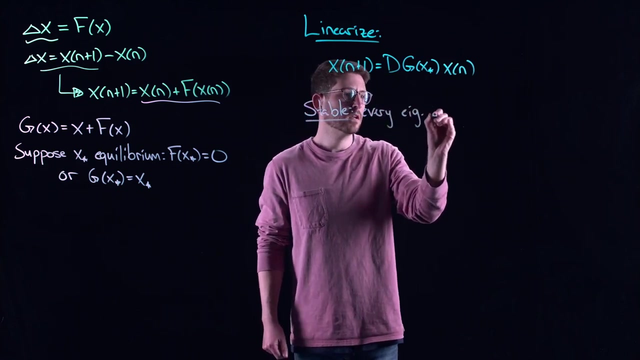 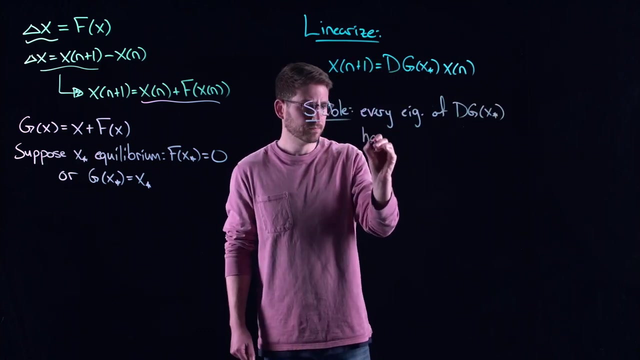 linear dynamical system and we have similar results to what we had in continuous time. So, in particular, all of the dynamics of this thing are determined by the eigenvalues of the matrix DG. In particular. we have stability if every eigenvalue, so every eigenvalue of DG of x star, has modulus, so modulus. 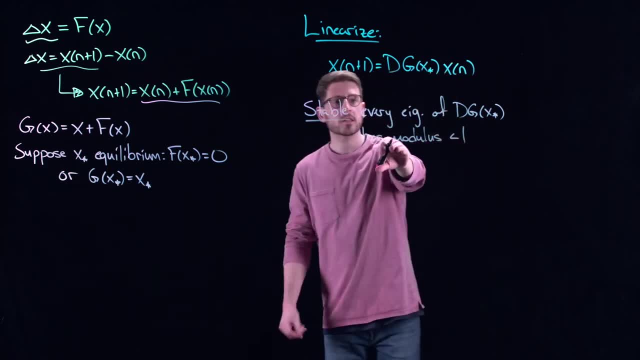 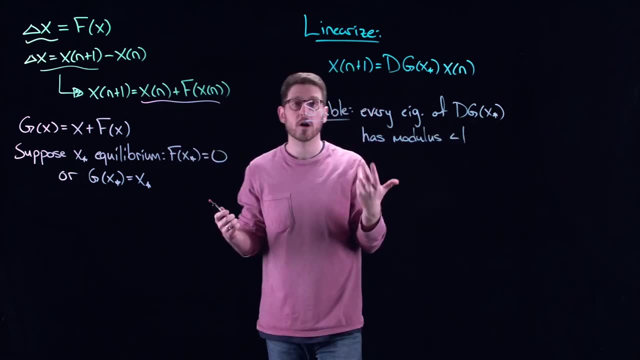 less than 1.. Now, the modulus here denotes the fact that it belongs to the unit circle in the complex plane. Remember, some of these eigenvalues could be complex conjugates of each other. The fact is, if you take the absolute value of a complex number, so they're. 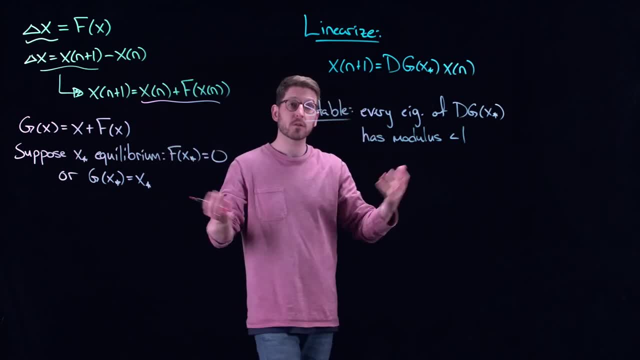 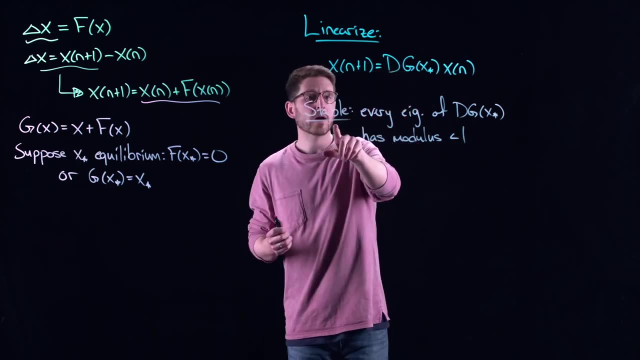 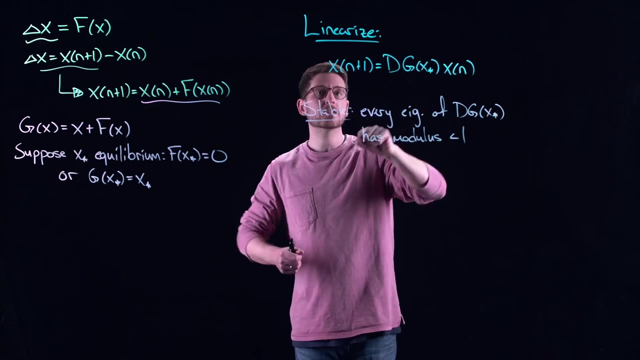 real parts squared plus the imaginary parts squared, all under the square root, the Euclidean norm. If every one of those eigenvalues is smaller than 1, then you have stability of your original equilibrium point. Why? Because we know that this Jacobian matrix actually becomes what's called a 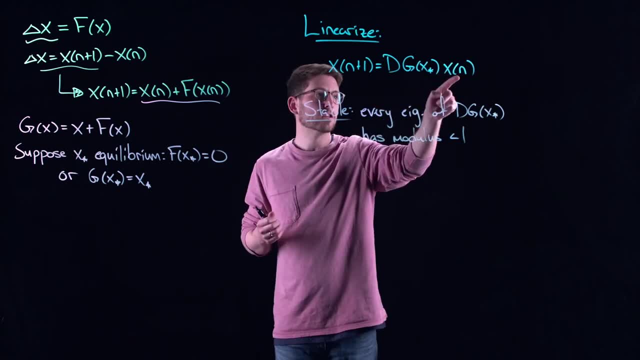 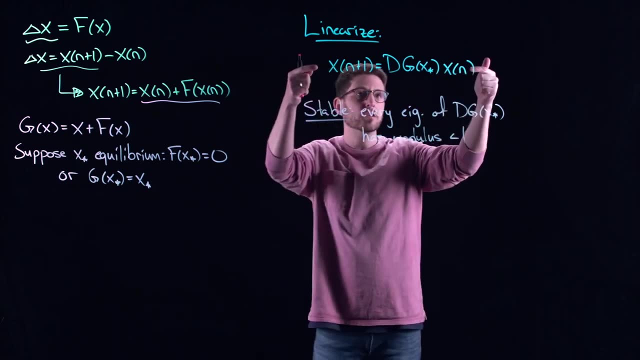 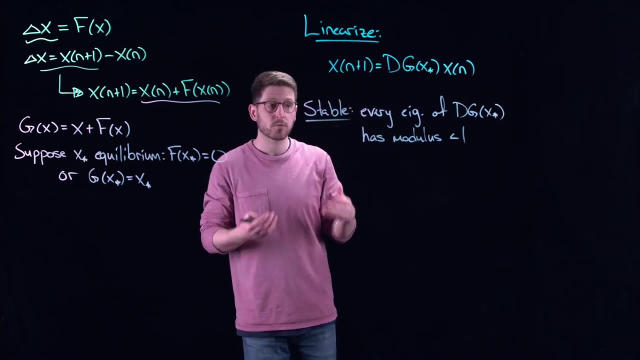 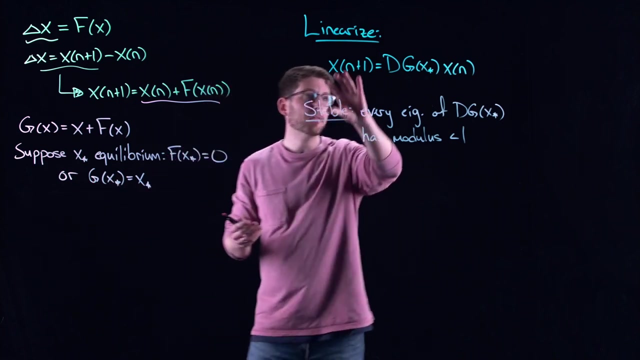 contraction. It says that after every iteration, so after each n you are contracting, you are getting smaller and smaller and smaller and smaller, until you disappear down to zero, as n goes to infinity. Now the stable manifold theorem that we learned for continuous dynamics is the same thing for these discrete time dynamics, If you 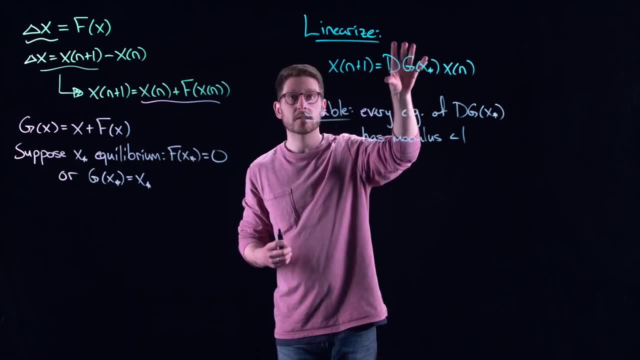 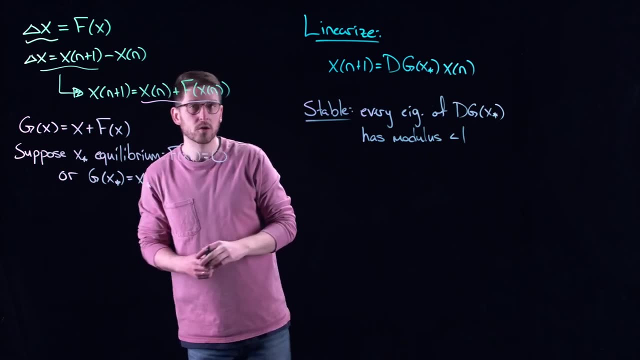 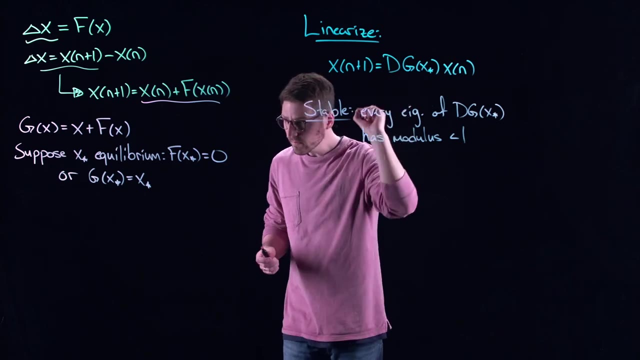 have a contraction for your linearized discrete system, then you find that local rectification is always continuous and if you have a contraction in this equilibrium then you have to contract gradually. So if you have a fully non-linear system, typically you have a contraction for your fully 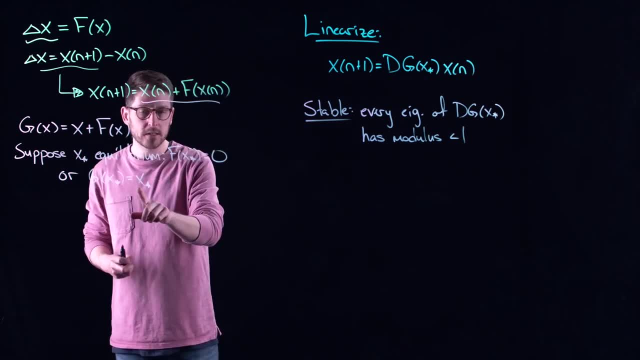 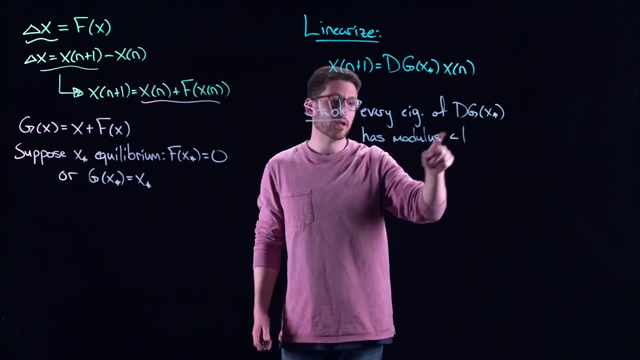 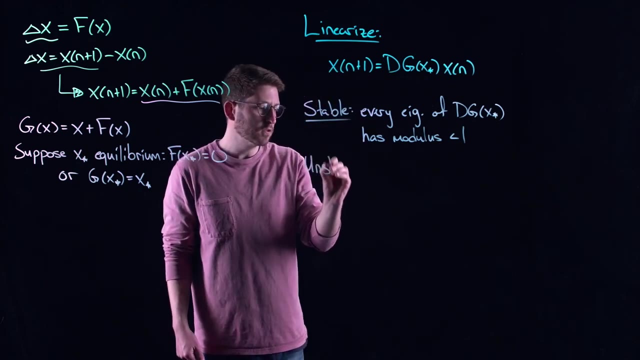 non-linear system. Remember, the local part comes in the fact that you're doing a Taylor expansion here and this tells you that if you start close to this equilibrium you are going to converge into it when the linearized matrix, the Jacobian, has all eigenvalues with modulus less than 1.. 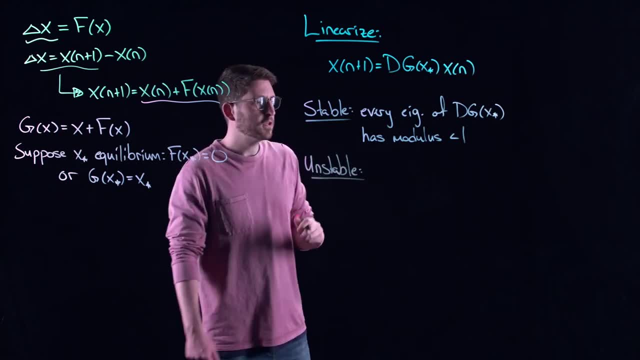 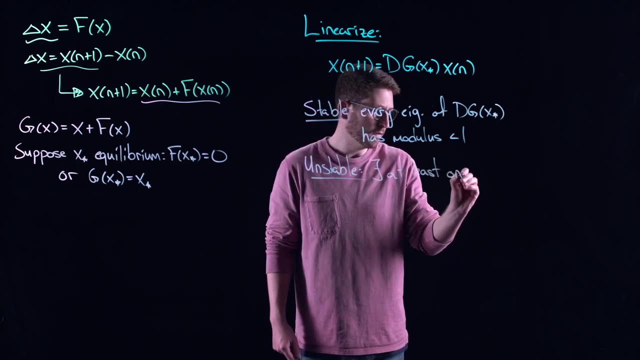 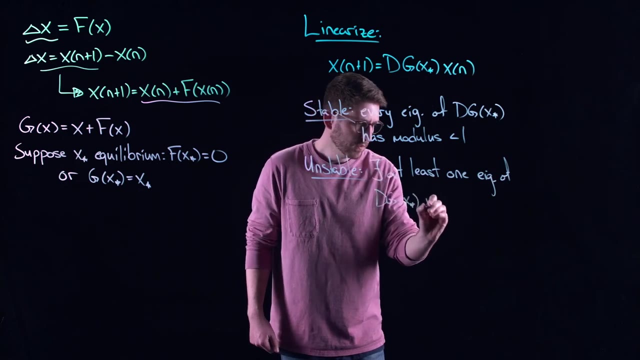 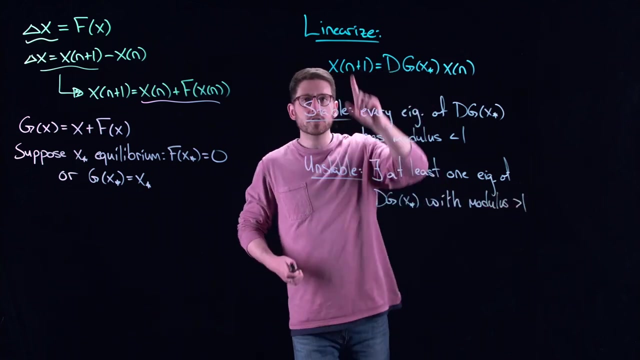 look at this the other way around as well. you can say that it's unstable if there exists at least one, so at least one eigenvalue of this matrix, dg of x, star with modulus, so modulus greater than one. So if there's even 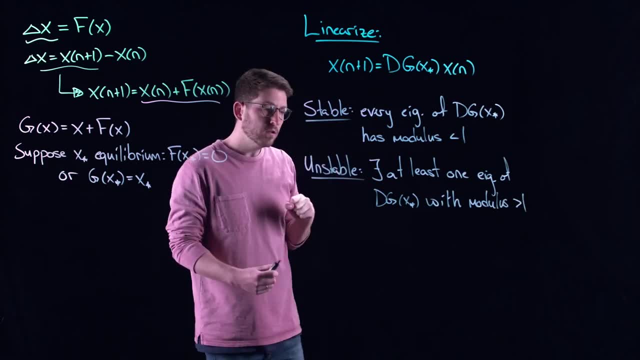 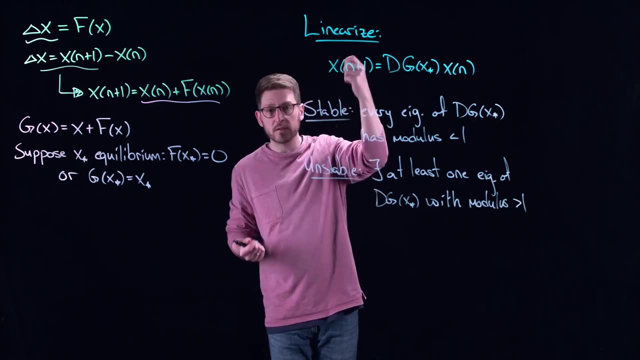 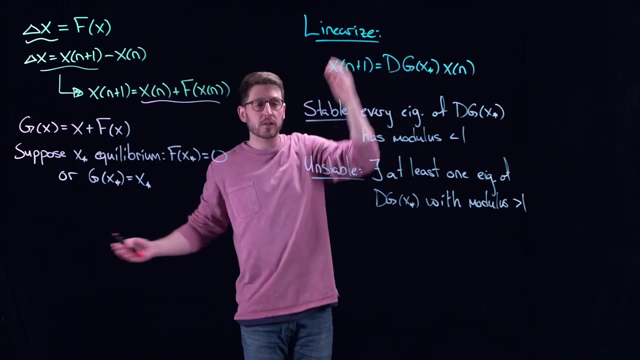 one eigenvalue outside of the unit circle, then you have instability. Why That eigenvalue? when you take successive powers of it, is going to get bigger and that means that you one dimension at least of this thing is expanding. You no longer have a contraction, you have an unstable. 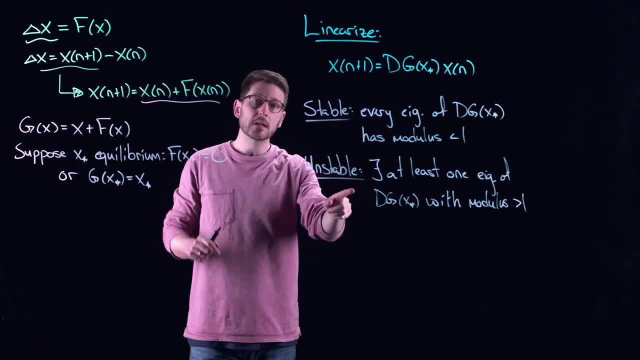 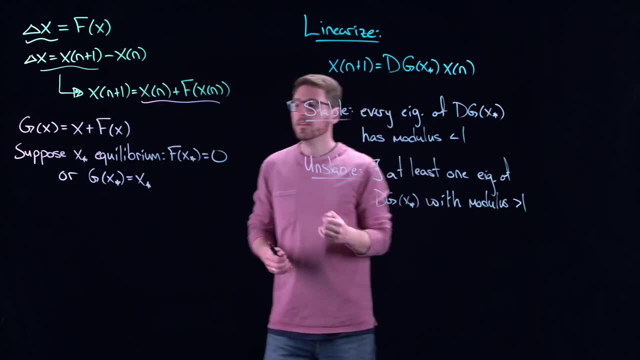 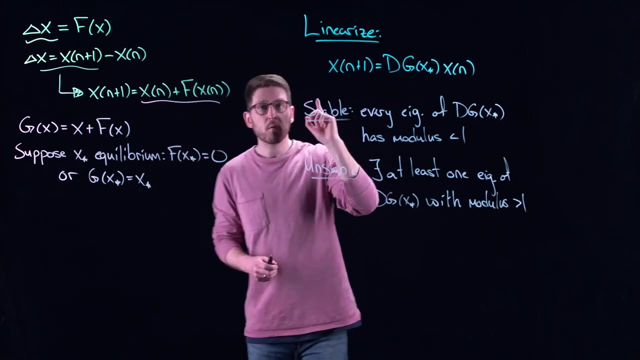 direction here and that instability from the linear system carries over into an instability for the non-linear system. That actually tells you that if you started close to this thing, then you would expect to be pushed away due to this instability. But what I really want you to notice here is it's the same basic process. 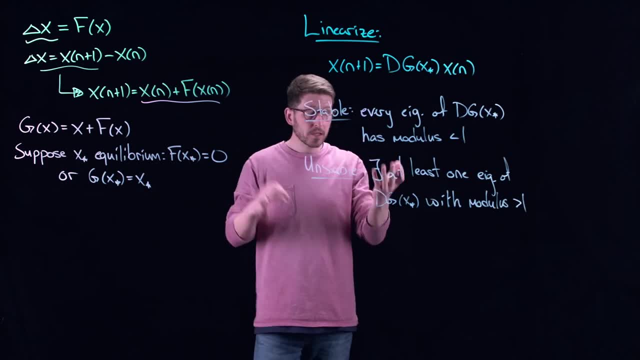 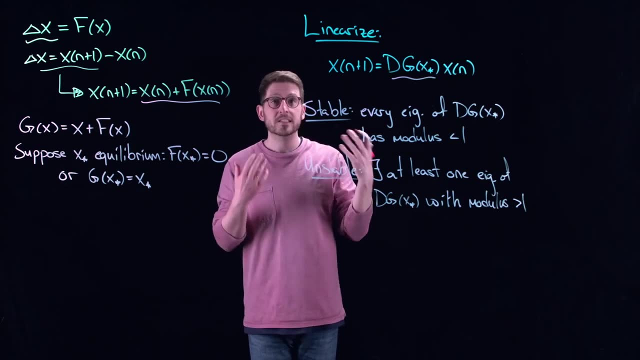 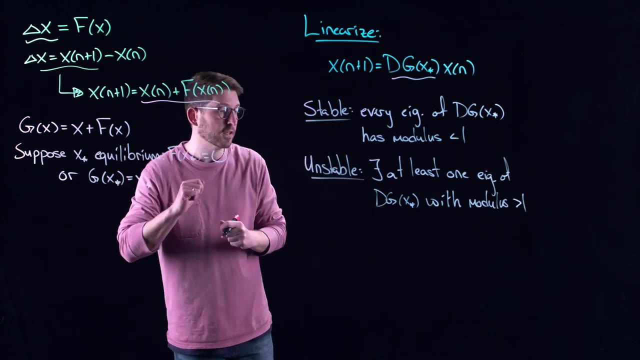 that we saw with continuous time, dynamical systems In particular. it all comes down to just analyzing the eigenvalues of a matrix. The stable manifold theorem tells you the same thing: If you have stability for the linear system, then it carries over to stability for the non-linear. 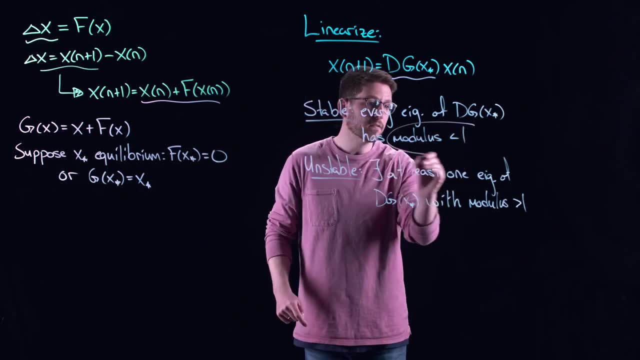 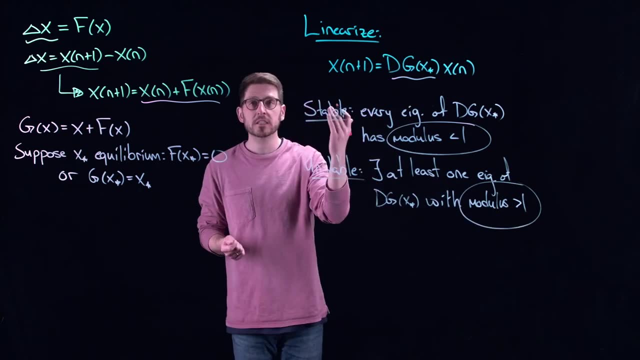 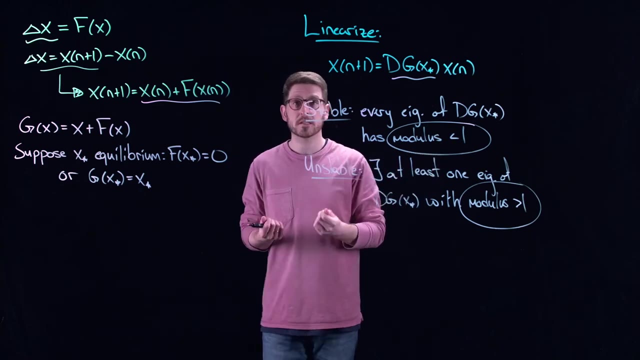 system. The only thing you have to be very, very careful of here is the meaning of stability is slightly different. For discrete time systems, you have to be in the unit circle in the complex plane. Remember, for continuous time systems you have to be in the left half of the complex.